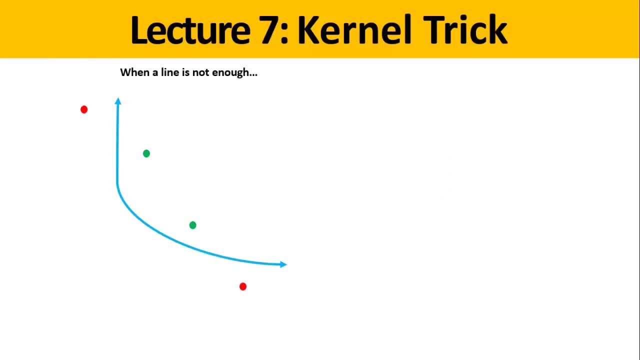 the box is drawing this line here, Or maybe we have to think outside the plane. If we found a way to lift the green point up, we can easily separate them by a plane. So what do you think is better, The curve on the left or the plane on the right? 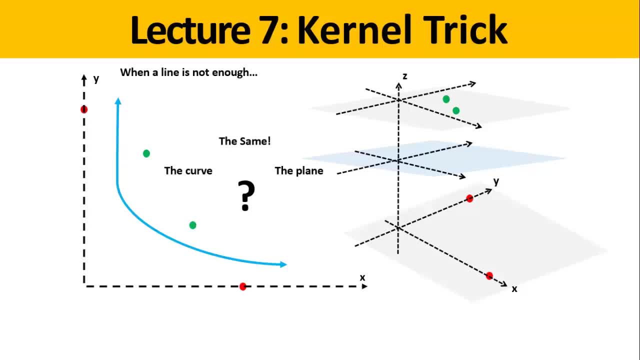 Actually, these methods are the same. Don't get confused. We're going to explore each one more deeper. Let's go first with the curve And let's put some coordinates on each point. We have this point, this one, the other green point and the last red point. 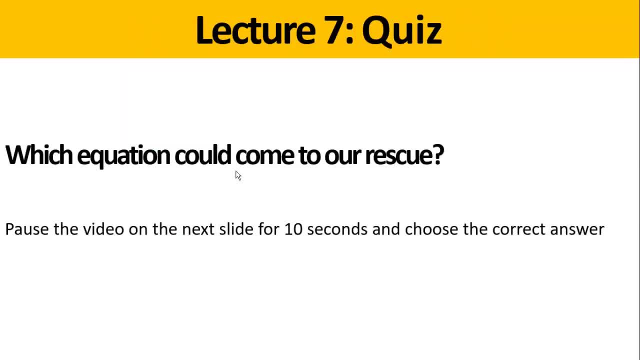 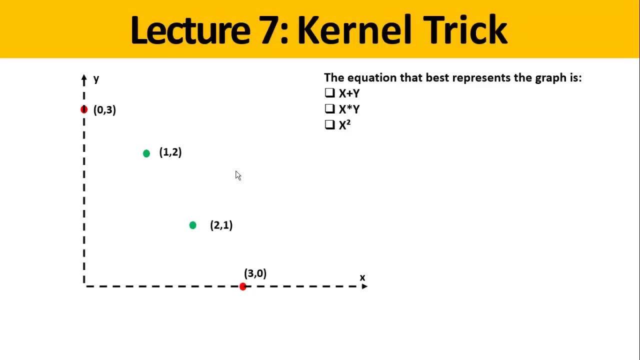 Ok, time for a quiz. Which equation could come to our rescue, in your opinion? X plus Y, the product X times Y or X square? This is not an easy question, so let's dive in into more details. We can draw a table. 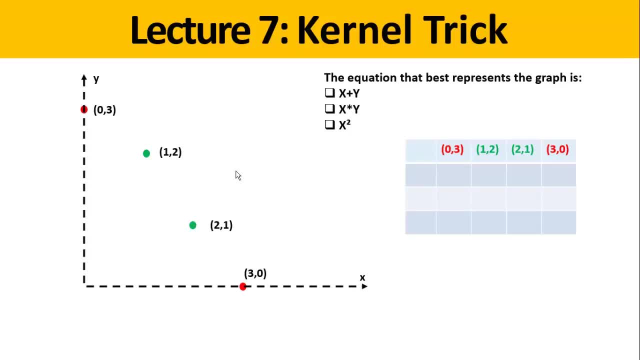 with the four points on the right. For the first one, X plus Y, we have. for the first point, 0 plus 3 is 3.. For the second one, 1 plus 2 is 3.. And for the third one, 2 plus 1 is 3.. And for the last one, the red, 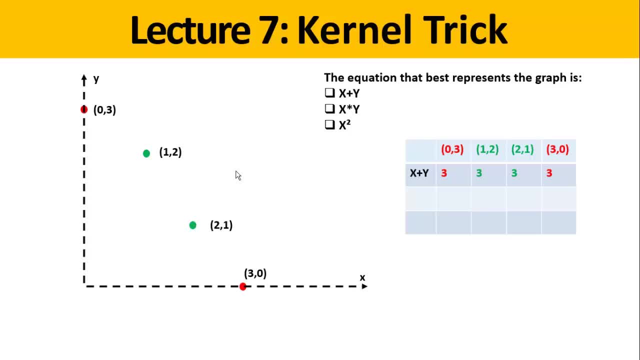 point, 3 plus 0 is 3.. With the second equation, the product For the first one, X plus Y, we have for the first one, 0 plus 3 is 3.. And for the second one, O five times 1 is 5.. And for the third one, 1 plus M minus A is 3. For 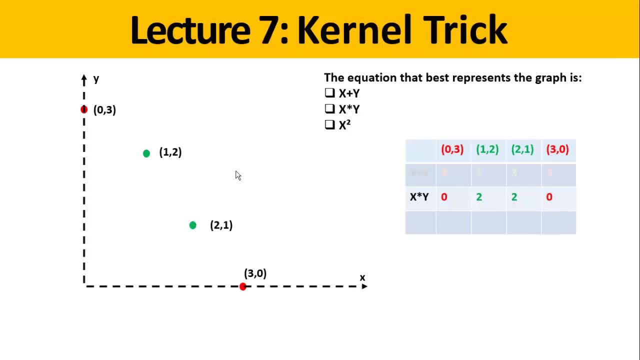 the first point we have 0.. And for the second one, 2 times 1 is 2.. For the third one, 2 times 1 is 2.. For the last one, 3 times 0 is 0.. 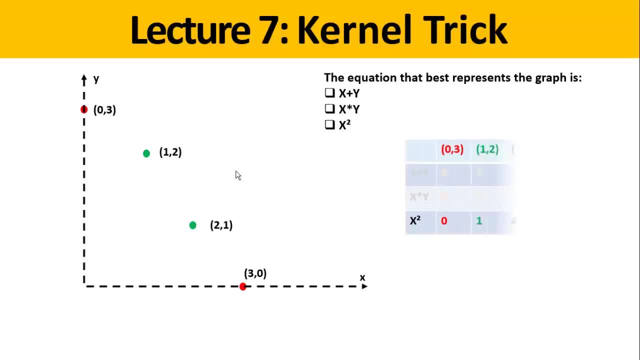 With the secret. you must find a lower value for the product by looking here For the last equation: X squared, the first coordinate square, 0 squared is 0, 1 squared is 1, 2 squared is 4, 3 squared is 9.. 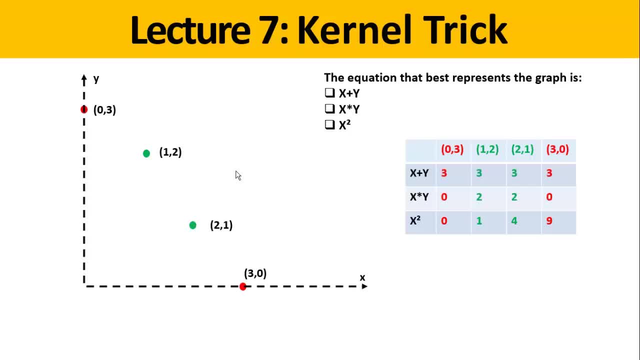 So if we look at two things, we can find an arbitrary number To do so. it would be If we look at the results of each equation. for the first one, it gives us 3 for all points. On the other hand, x squared gives us 0,, 1,, 4 and 9.. 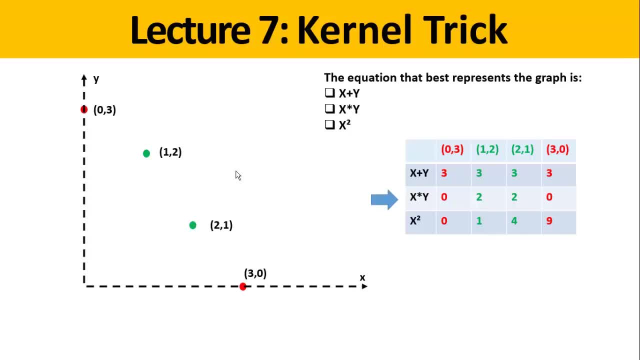 But if you look at the product x times y, it gives us 0 for the red points and 2 for the green points. So that's what we was looking for: An equation that gives us big values to the green points and smaller values for the red points, or vice versa. 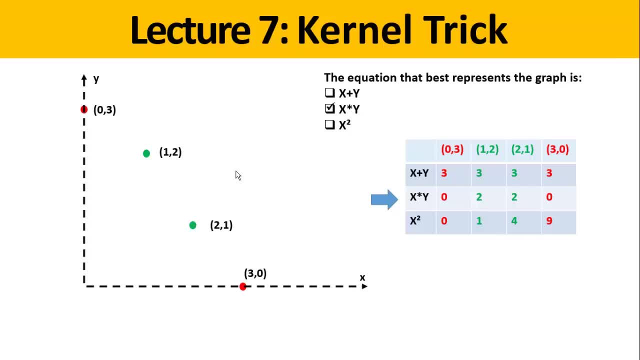 So we're going to use this equation. That was the right answer. Now let's put the results on the graph. You can see that for the red points we got 0 for each one, And for the green points we got x times y equals 2.. 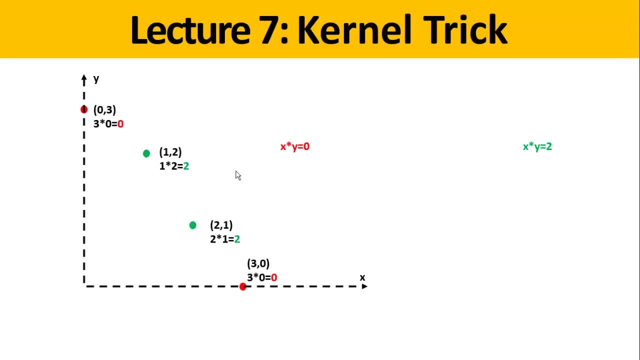 And what separates 0 and 2? It's 1.. And what is? x times y equals 1? It's exactly: y equals 1 over x, which is the equation of hyperbola that you can see here. We can use the same function, x times y, to put the points on another plane. 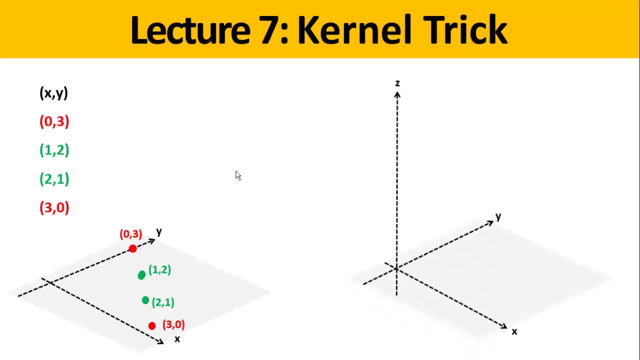 So for a 3D representation we can use the coordinates x, y, x times y. In this case the coordinate of the first point, 0,3, will become 0,3,0.. And the point will be here. 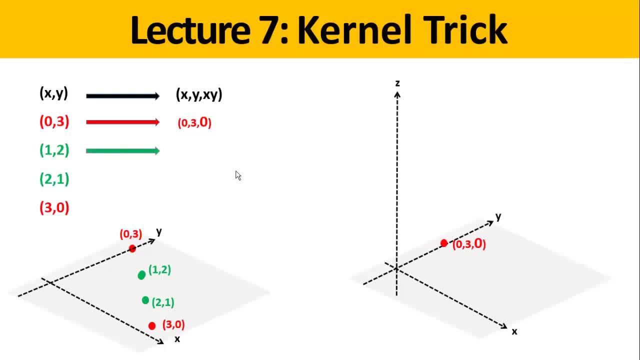 For the second point, the first green point- the coordinates will be 1,2,2.. And it will move up. For the third point, the coordinates will be 2,1.. And it will also move up. The last point- 3,0, will have the coordinates 3,0,0. 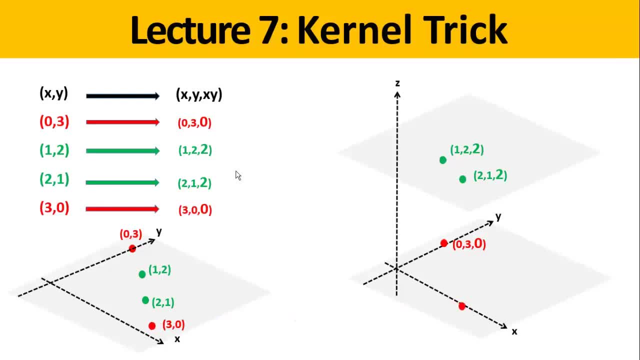 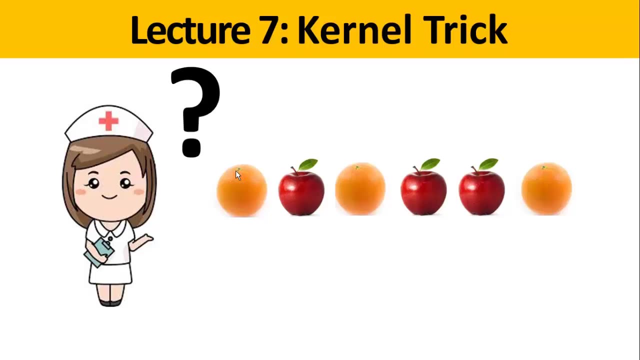 And it will be here. Now you can see that we have separated our points with the plane, And this is exactly the kernel trick. You can think of it as a surgeon who is looking to separate apples from oranges, And she got an idea.